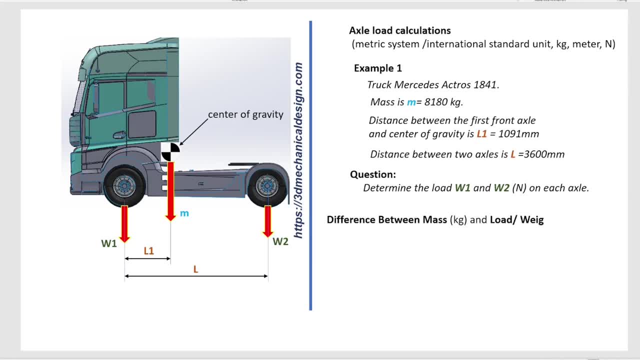 Difference between mass and load weight. The mass of a body is the amount of matter contained within it, While the weight of a body is the force acting on it due to acceleration, due to gravity. Mass of the International Standard Unit of Mass, or the SI unit, is the kilogram. 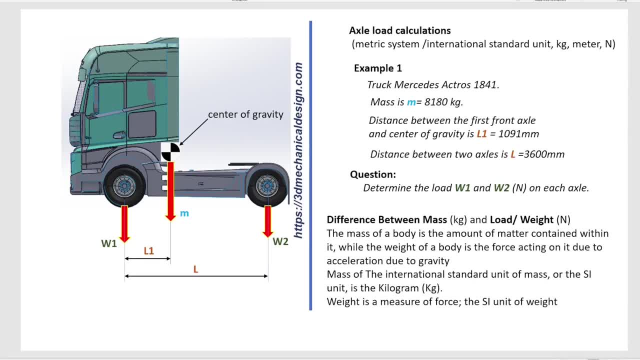 Weight is a measure of mass. When a force has a mass of 4 gibinent acting on it, the function of this mass is pressures, or fun waking, the direction it is responsible for. When a force passes through it's spin diameter, theации trumpet of mass is controlled by Newton. 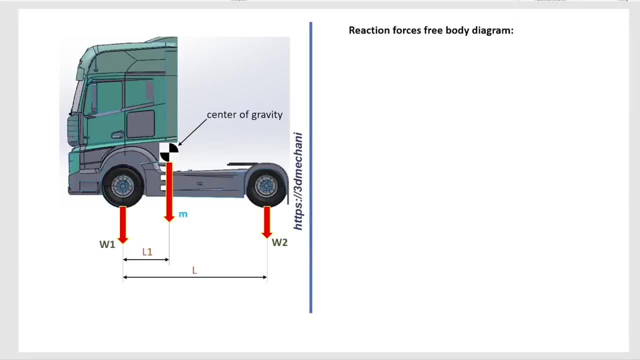 333!. In theères and piece of the vol� of force, the SI unit of weight is Newton, arising from the Reaction forces- free body diagram. Reaction forces- free body diagram. Reaction forces- free body diagram- F reaction forces. The first equilibrium condition for the Vector sum of the external forces on the rigid object must equal zero. 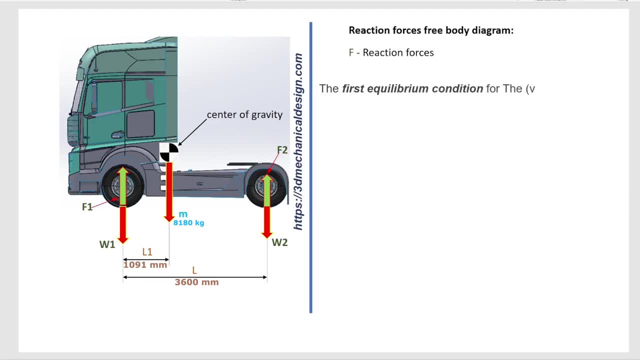 The sum of the F equals zero. F1 plus F2 minus F3.. F1 plus F2 minus F3.. F1 plus F3.. The vector must also have a force relationship. calls out F1 minus F3.. minus FM equals 0 according to Newton's second law of motion. 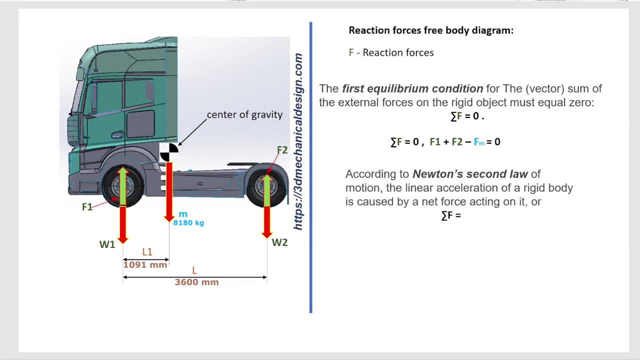 the linear acceleration of a rigid body is caused by a net force acting on it, or. F equals M times G. G acceleration due to gravity is 9.806 meters per square second. FM equals 8180 times 9.806 equals 80,213.1 Newtons. 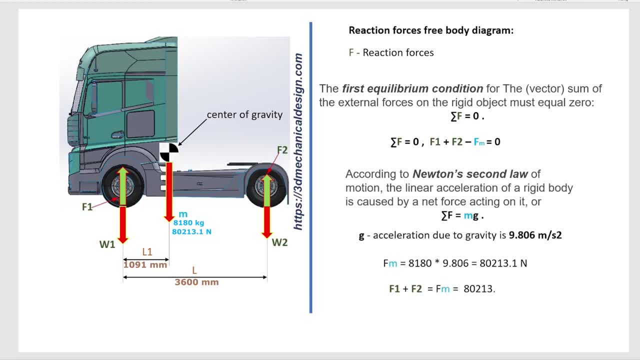 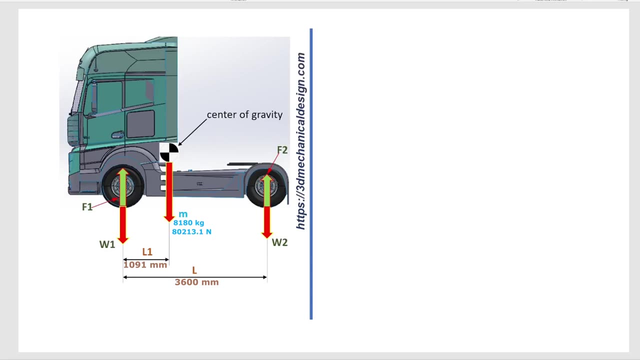 F1 plus F2 equals FM, equals 80,213.1 Newtons. F2 equals 80,213.1 minus F1. second condition of equilibrium: the sum of all external the moments of forces, torques from external forces is zero. so the condition that all the moments of forces acting on the body is zero leads. 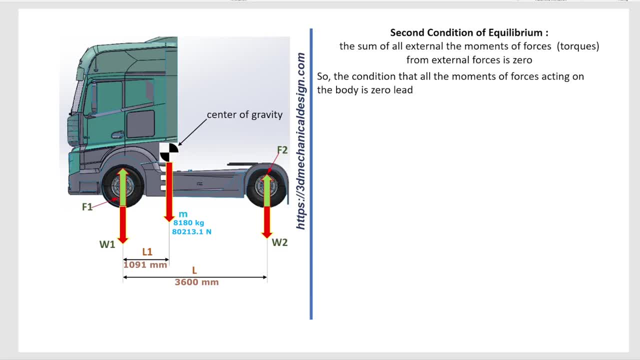 us to the equation: the sum of the M equals zero. the sum of the moments M from center of gravity equals zero. MF1 plus MF2 plus MM equals zero. MF1 plus MF2 plus MM equals zero. MF1 plus MF2 plus MM equals zero. M F1, equals F1, times L1. 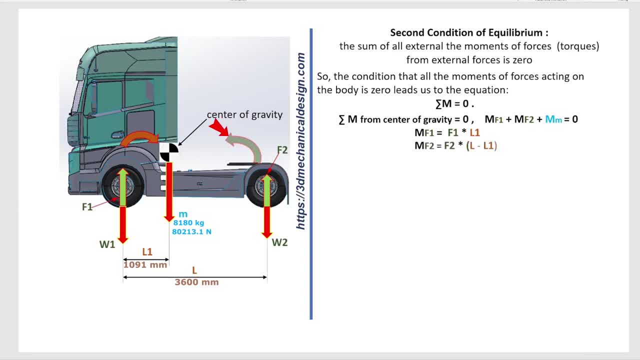 M. F2, equals F2, time L minus L1.. M. M equals M. times 0 equals 0.. F1, times L1, equals F2, times L minus L1.. F2, equals 80213.1, minus F1. 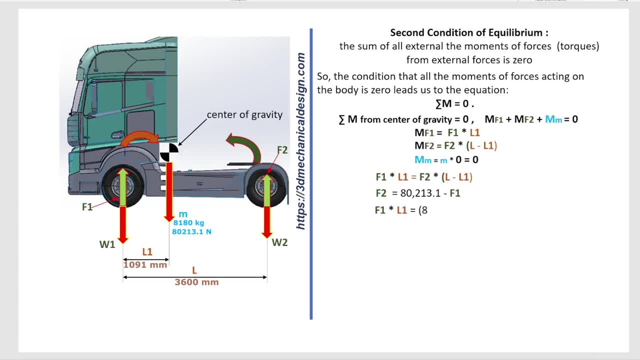 F1, times L1, equals 80213.1, minus F1, times L minus L1.. F1, times 1091 equals 80213.1, minus F1, times 3600 to 1091.. 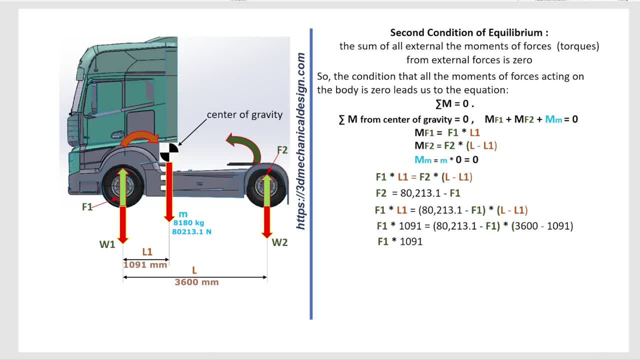 F1 times 1091, equals 80213.1.. 80213.1, minus F1, times 2500, and 9. F1, times 1091, equals 201254667.9, minus F1, times 2.509.. 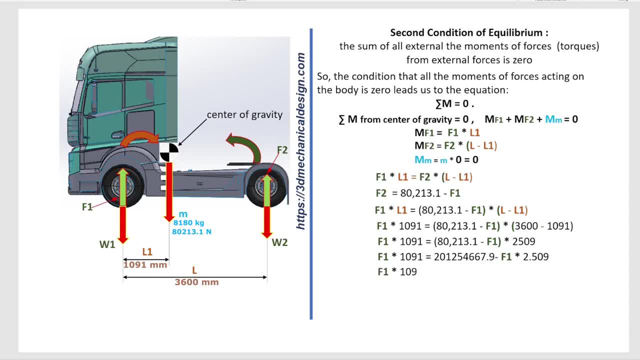 F1, times 1091, plus F1, times 2.509 equals 201254667.9.. F1, equals 201254667.9,. divide 3600, equals 55900, and 4 newtons. 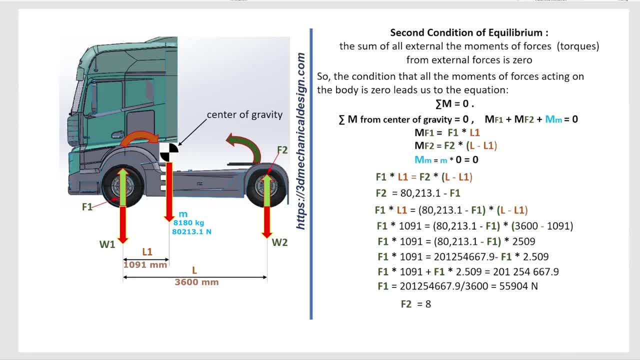 F2, equals 80213.1, minus F1, equals 80213.1, minus 55904.. F2, equals 24309.1 newtons. W1, equals F1, equals 55904 newtons. 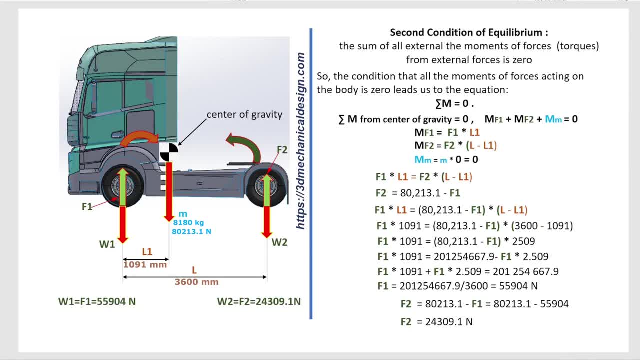 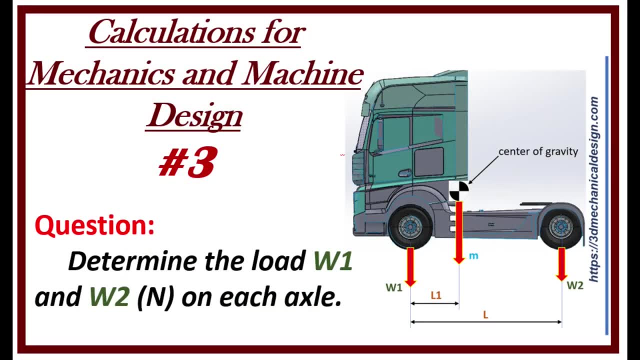 W2, equals F2, equals 24309.1 newtons. I hope you will find this video useful. If you want to continue to improve your design skills and see more of our video, please subscribe to more content like this in the future. Thank you for watching.